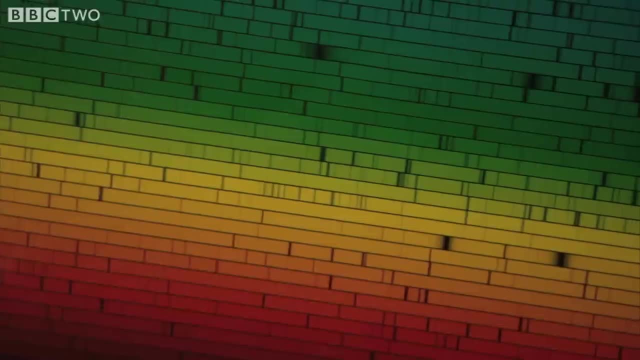 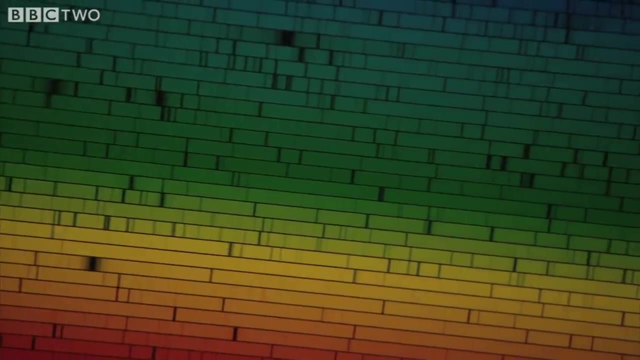 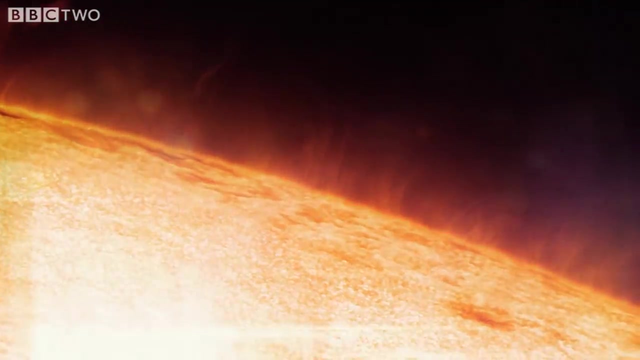 It's the spectrum of the light from the Sun in the sky, But if you look a bit more closely, then you see that this spectrum is covered in black lines. These are called absorption lines. Each element within our Sun not only emits light of a certain colour, it also absorbs light of the same colour. 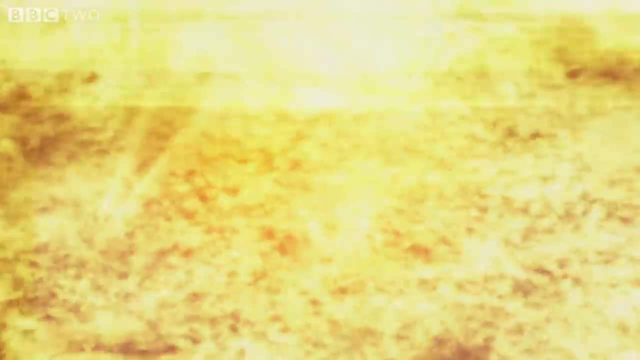 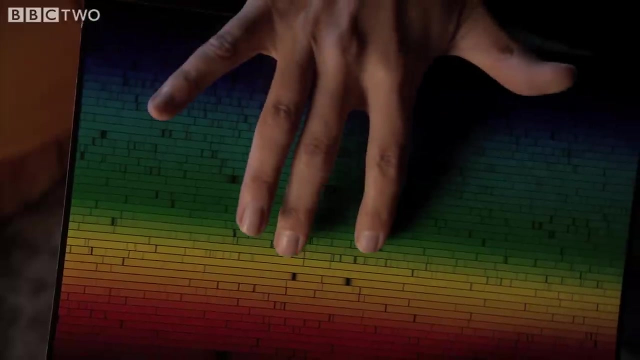 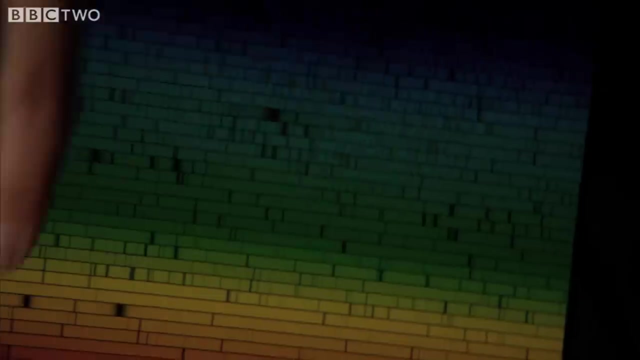 By looking for these black lines in the Sun's light. we can simply read off a list of its constituent elements like a barcode. For example, these two black lines in the yellow bit of the spectrum are sodium. You can see iron Right down here. you can see iron. 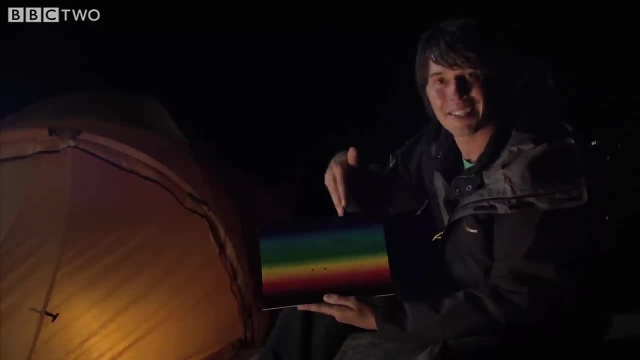 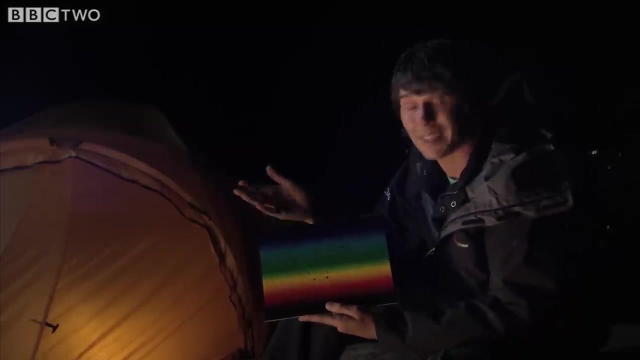 And you can see hydrogen. So by looking at these lines in precise detail, you can work out exactly what elements are present in the Sun, And it turns out that that's about 70% hydrogen, 28% helium and 2% the rest. 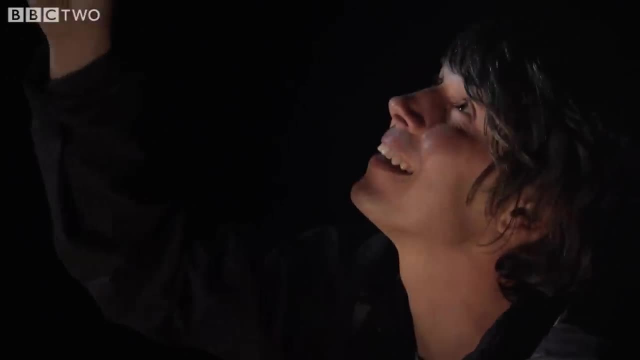 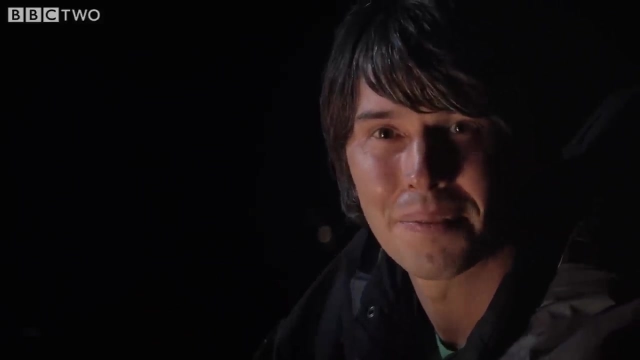 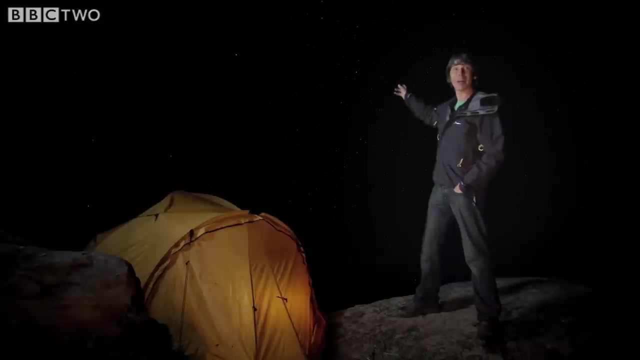 And you can do this not only for the Sun but for any of the stars you can see in the sky, And you can measure exactly what they're made of. So that star there is Polaris, the pole star, And you can see that because all the other stars in the night sky appear to rotate around it. 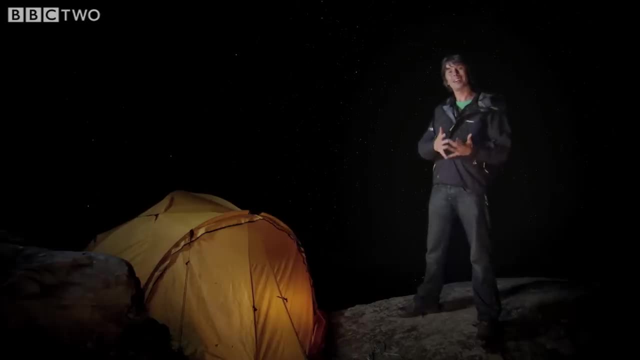 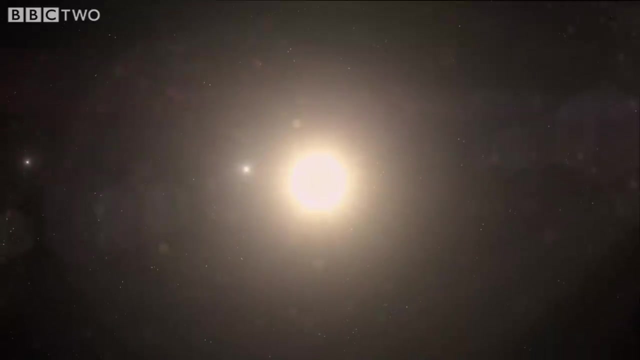 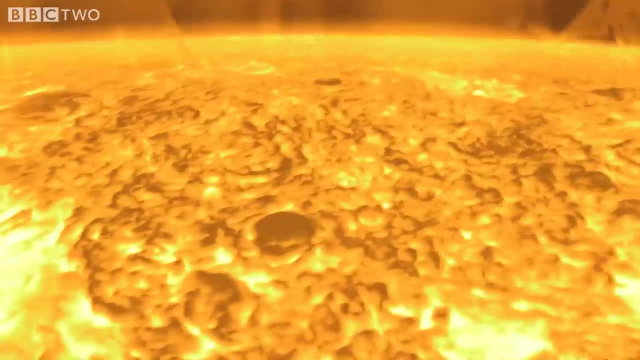 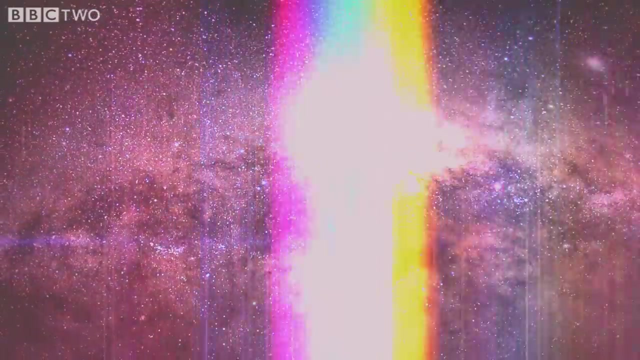 Now it's 430 light years away, But we know just by looking at the light that it has about the same heavy element abundance as our Sun, But it's got markedly less carbon and a lot more nitrogen, And the same applies for other stars. 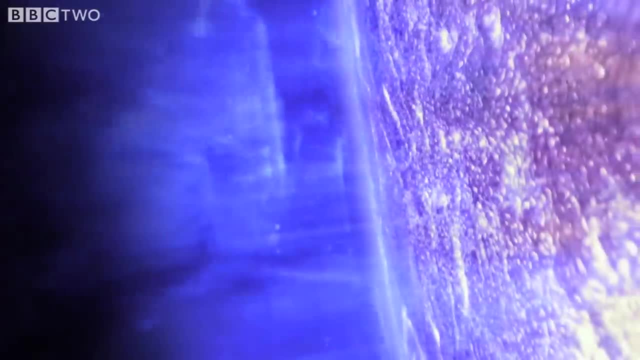 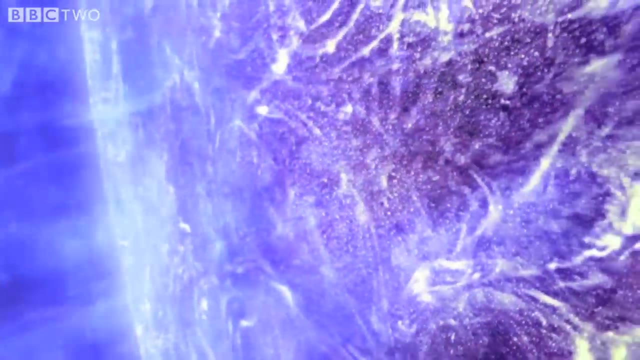 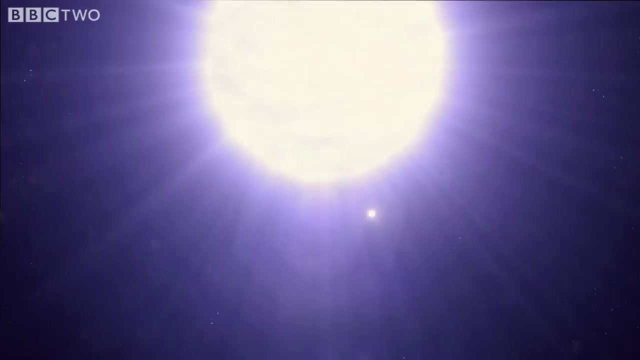 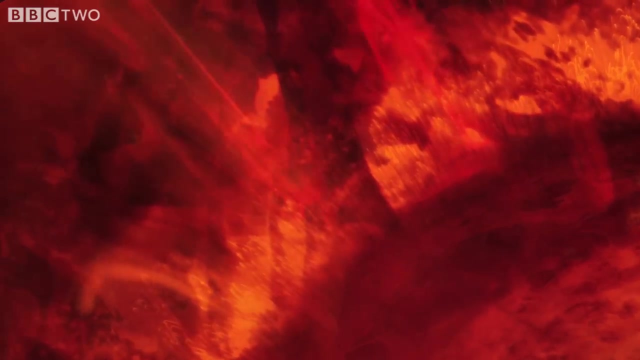 Vega, the second brightest star in the northern sky, has only about a third of the metal content of our Sun, Whereas other stars are metal heavy. Sirius, the dog star, contains three times as much iron as the Sun, And Proxima Centauri is rich in magnesium.